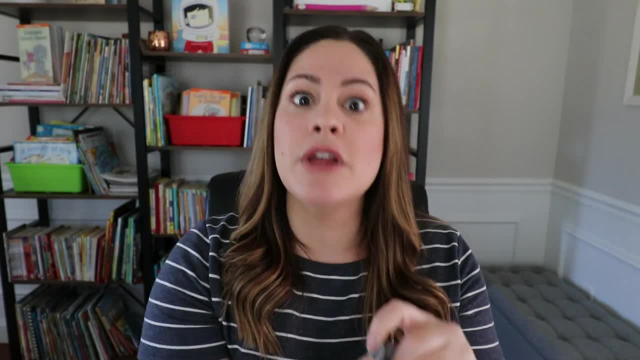 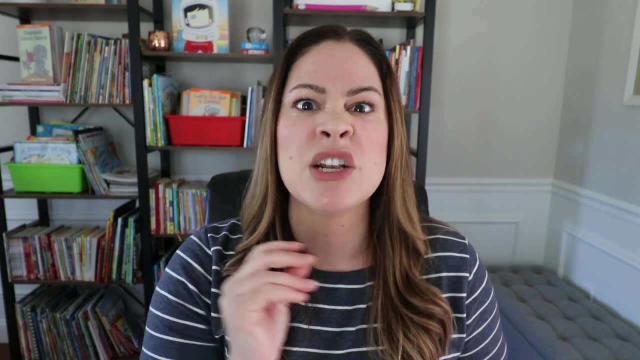 magnet tape on the back of it. So the front is showing. And then also I'll make sure some have the magnet tape on the front, So the back is showing. So students get familiar looking at both sides and quickly being able to recognize if that is a quarter, a nickel, a dime, et cetera. 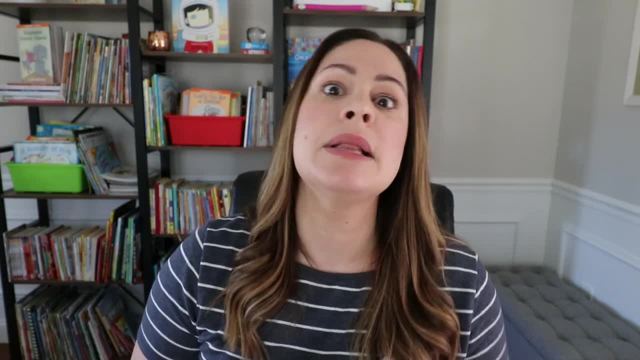 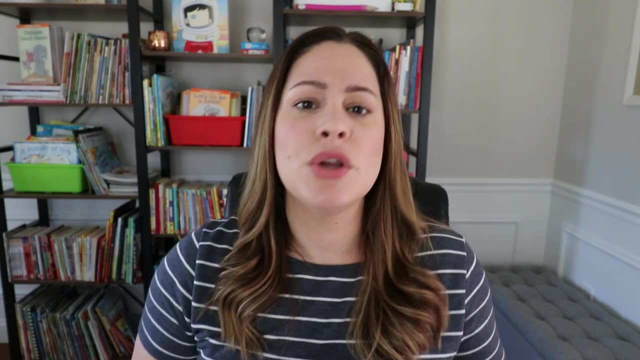 Now to do this, I will basically use those anchor charts and I will give students plenty and plenty of time holding, feeling, touching and examining all different types of coins You can find play money pretty cheap. I will go ahead and link the ones that I use down in the description. 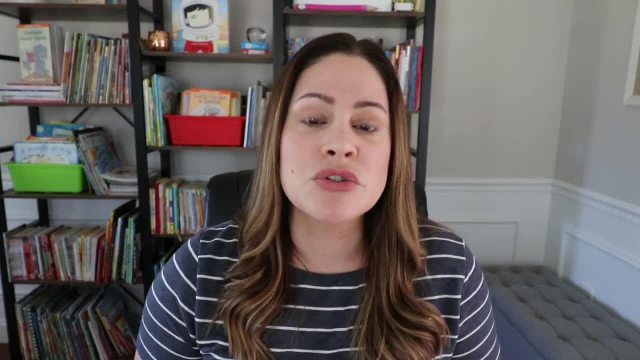 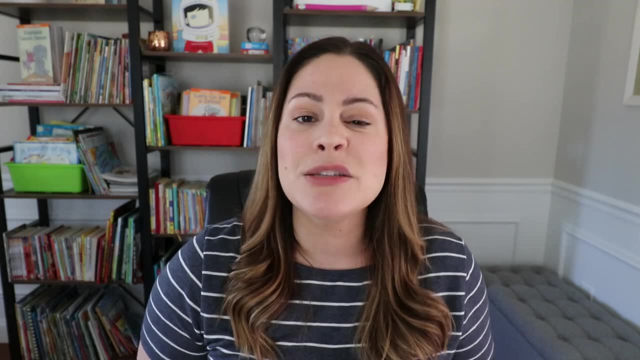 But if you don't want to buy- you know fake money- or if you don't have some in your classroom, definitely write a little note home to parents, maybe a week or two before you're about to start a money unit, and ask them if they can send in some coins, just a bag of coins. they have laying 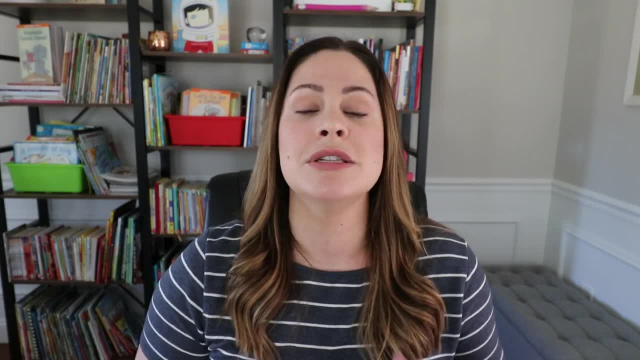 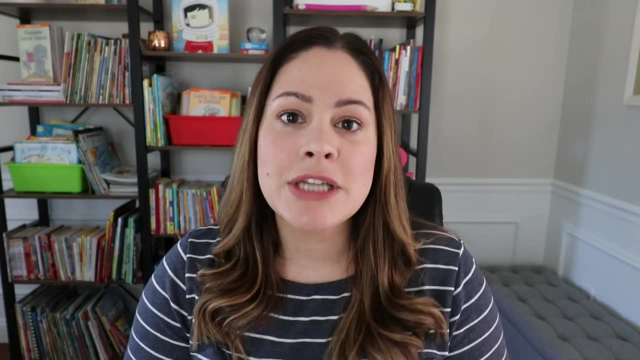 around the house. That way you can take them and you can sort them so your students can have them And, like I said, they really need to touch them, feel them, see them, to be able to identify them during this stage, Each day, throughout our money unit. 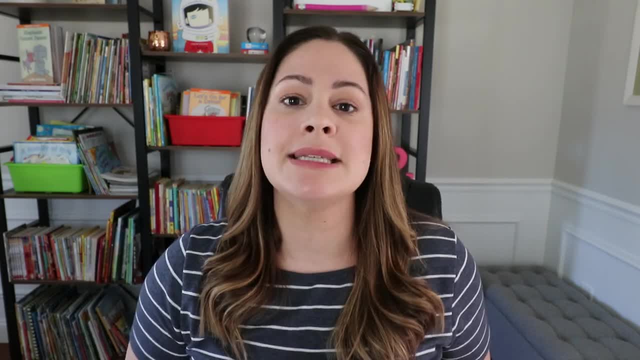 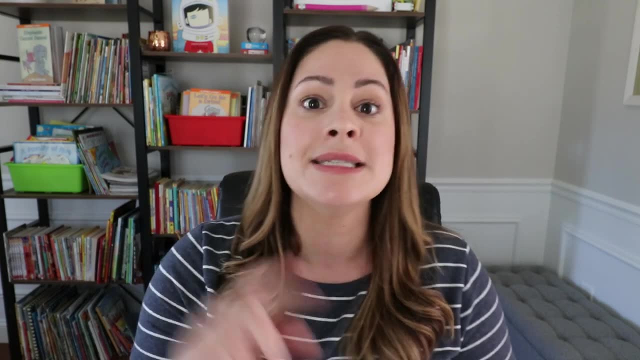 we have students use those coins up on the board The first couple of days. I may choose to put you know six or seven different coins up there And I will simply have students come up, choose one of the coins, identify what it is, identify the value and then put it with the 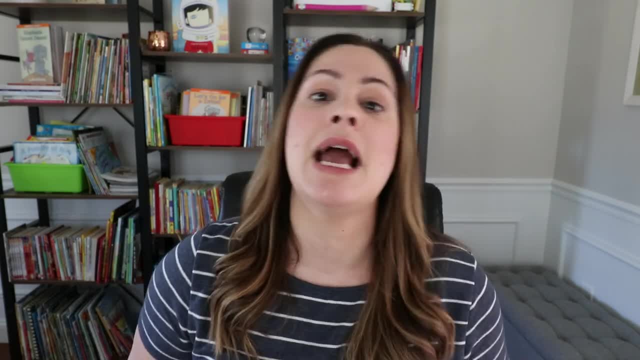 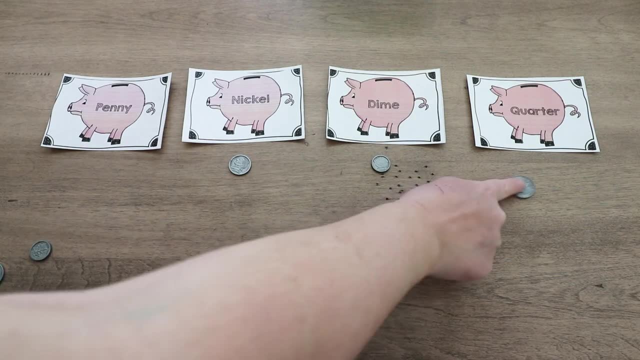 anchor chart For a more independent or partner activity. I also like to have students use little headers like this one right here, And I like them to be able to kind of grab a little bag and they can go ahead and sort those coins on their own. All right, once your students are readily able to. 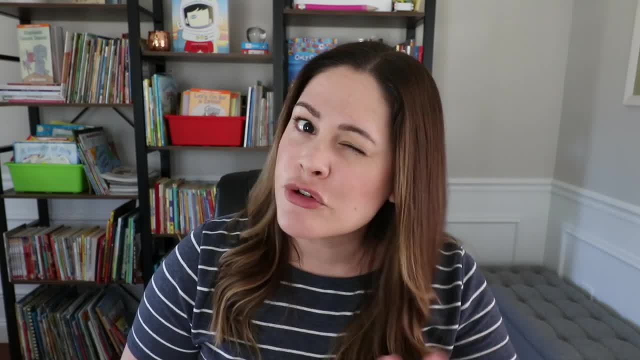 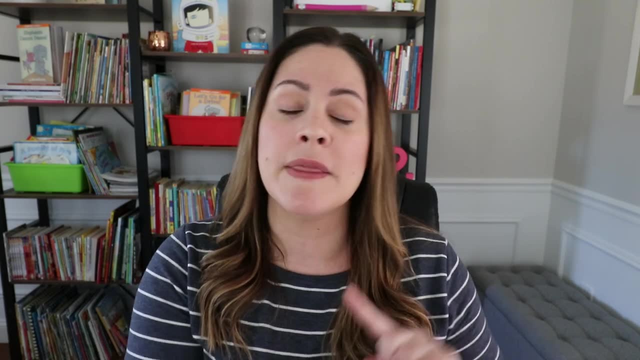 identify the different coins and their values and, even if they're not 100% proficient with that yet, that's something you'll review throughout this unit- And, like I said, each morning or each day with those coins on the board, make sure students are really seeing them, and just quickly. 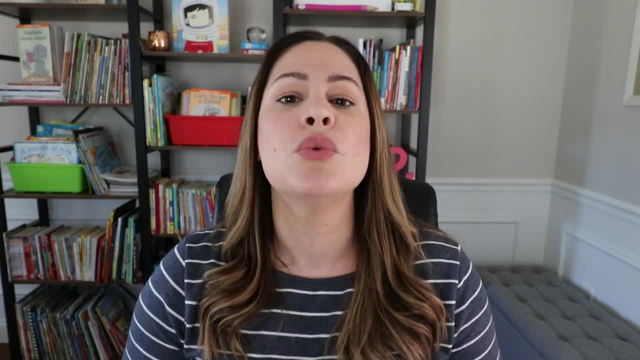 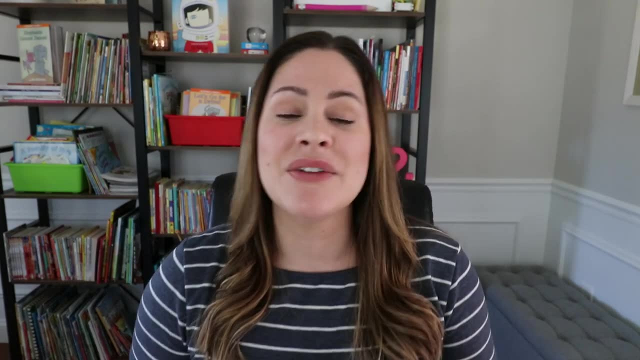 identifying and reviewing them all the time After they've gone ahead and do that. you want them to be able to get used to counting up those coins to find a group's value, And when doing this, I definitely have students count the same type of coin first. So when we're practicing, 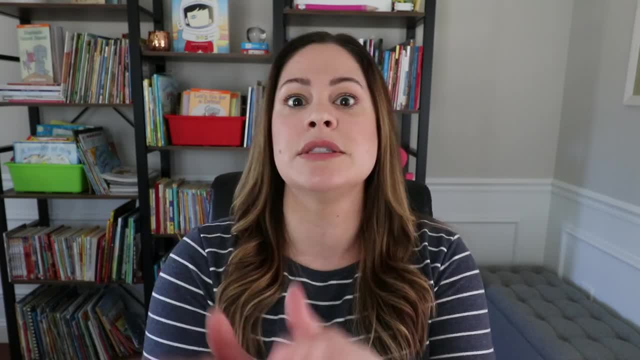 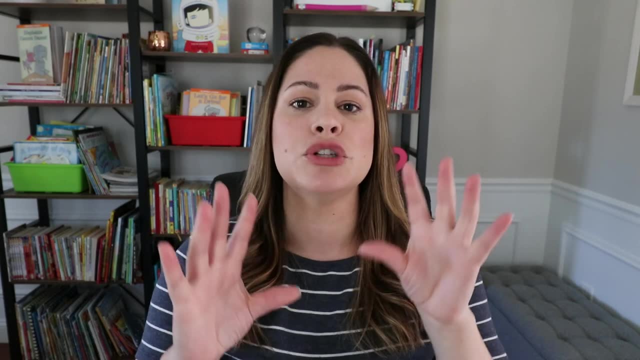 skip counting when they're counting up the values. I will only give them some groups of nickels to count first, and then groups of dimes and then groups of pennies and quarters. This helps students really quickly be able to actually see the different types of coins, identify what it is. 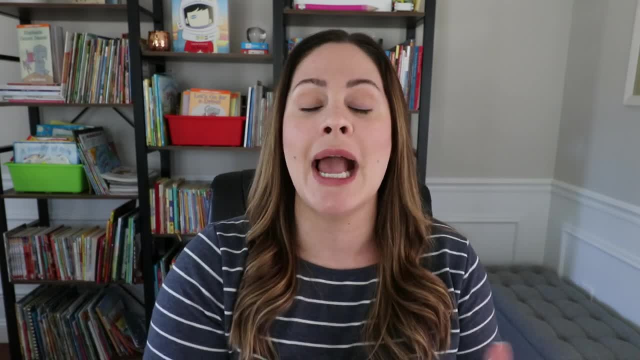 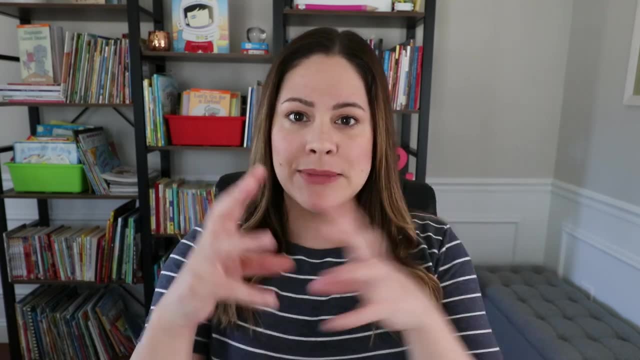 know the value in their head and then start their skip counting to determine how much value they have with that many coins. Your students are pretty familiar with skip counting, so being able to count up those same set of coins should be pretty quick for them Only after they've done. 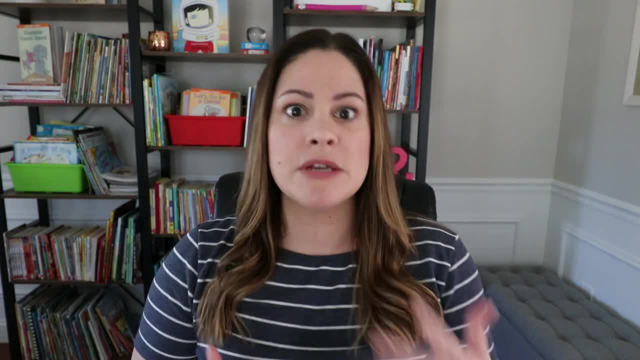 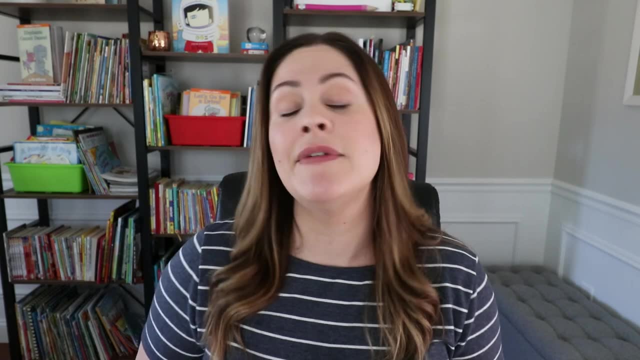 that will they be able to get used to it. So I'm going to go ahead and start by going on to teaching students how to count up mixed groups of coins, And when doing that, I take a few different steps. First, I have students go ahead and look at the group of coins they have and sort them by type. 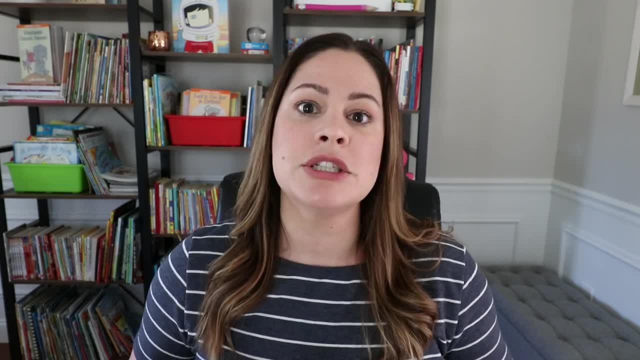 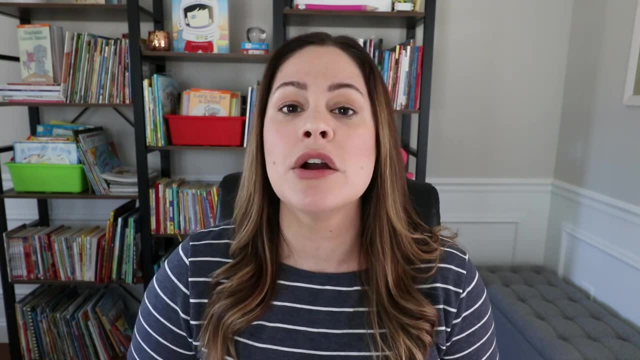 So once they're sorted by type, then I will have students count up the coins with the largest value first. So if they have any quarters they will start there. Then we go in descending order to make sure they count up the dimes. if there are any, then the nickels, then the pennies, Some of 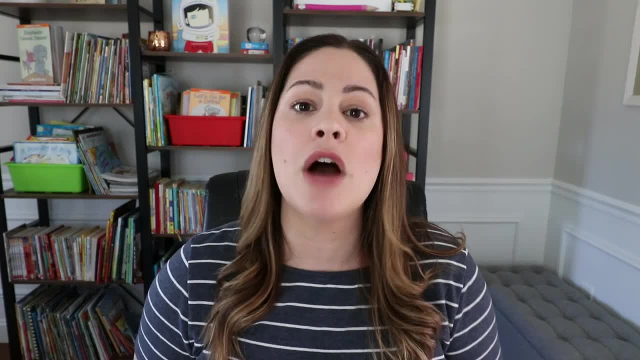 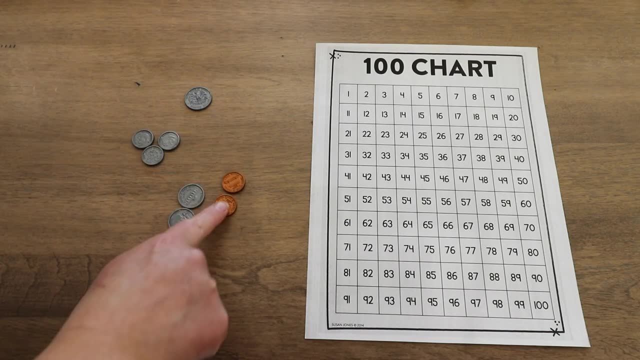 the students might be able to get this pretty quickly, but if they don't, I always like to offer a 100 chart So students can go ahead and, like I said, if they have those quarters and they know it's 25, they can go ahead and put their finger right on 25.. And then, if they see some dimes, 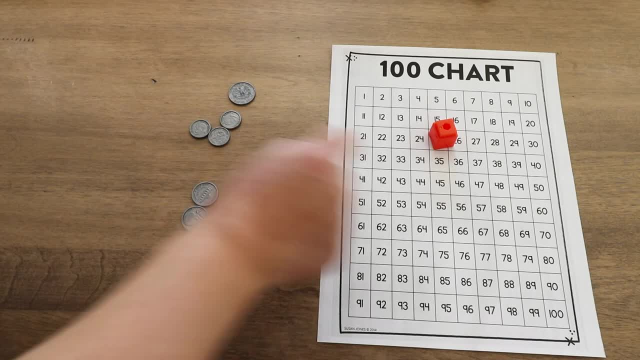 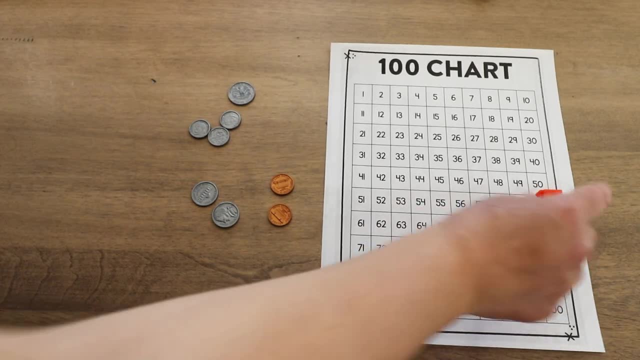 they know already to skip count down the 100 chart, two or three depending on how many dimes there are. Then they can go ahead and count the five for nickels and then the pennies. they just add on each one. As with any new skill, this is absolutely something I would model a few times. 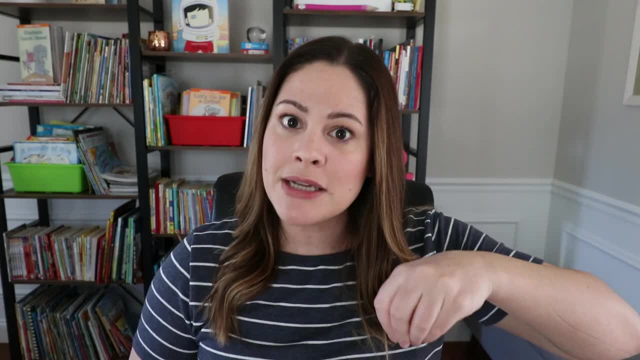 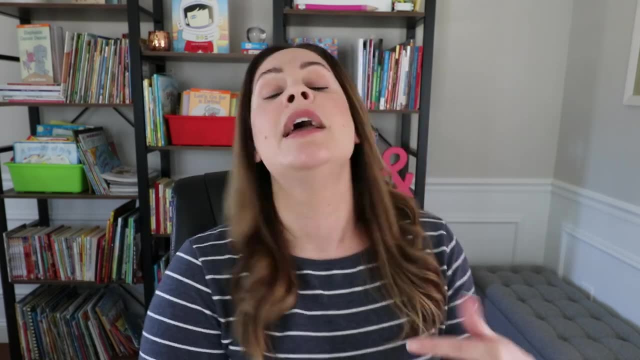 and then I would go ahead and give students little baggies of coins And I'd probably have them do this with a partner first, so they can kind of work together and use that 100 chart if they need to. And I would give them a little bag of coins And in first grade I would make sure 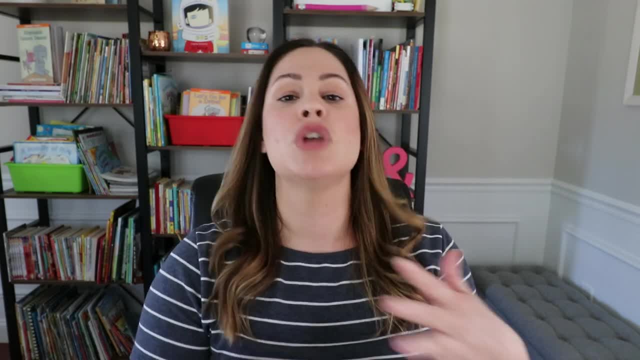 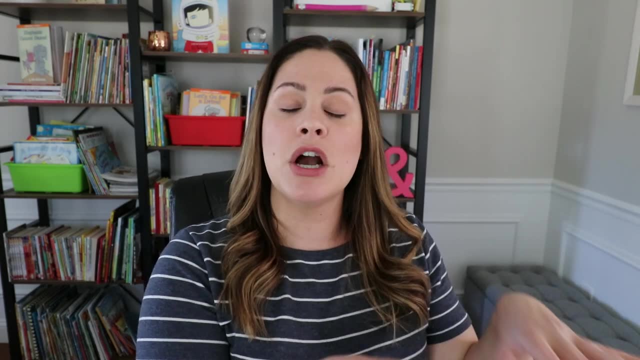 that the value of each bag does not go over $1. So you might want to make 10 to 20 different little bags, put them together and then just pass it to a group of students And after they've gone ahead and figured out, counted up the value of that bag, they can put it back together. 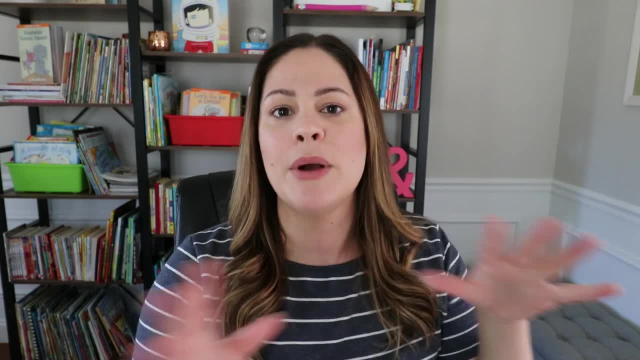 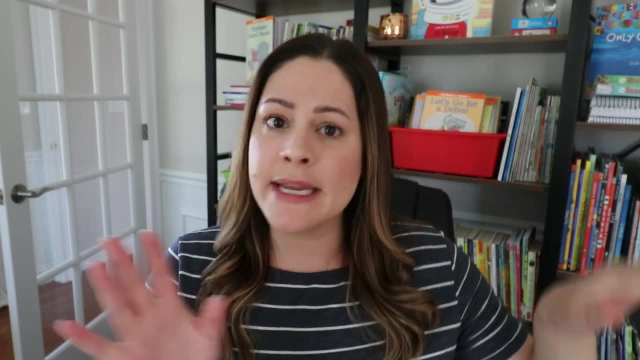 In trade with another group. you can collect them all, switch them up however you want to do it, but have them practice doing that quite a few times. Okay, so now students are familiar with the coins, And those anchor charts I shared at the beginning are something I absolutely keep up. 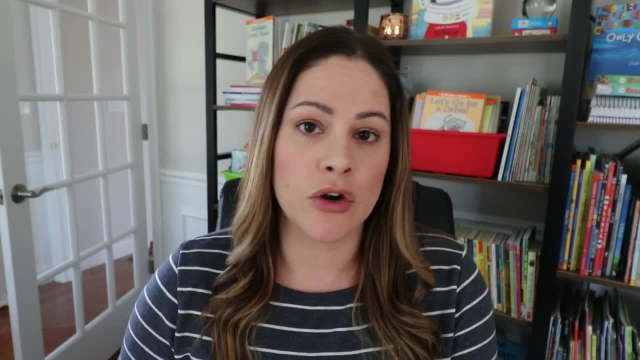 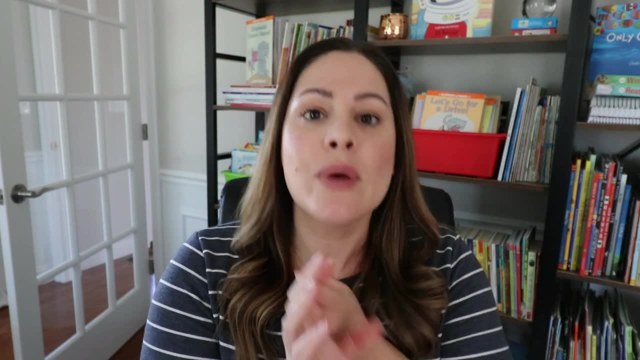 throughout this entire unit and pretty much for the rest of the year, if you didn't already have them up. But that way students can go ahead and reference them whenever they get a little tricked up, So they can quickly identify the coins and their values. And now they're getting pretty good. 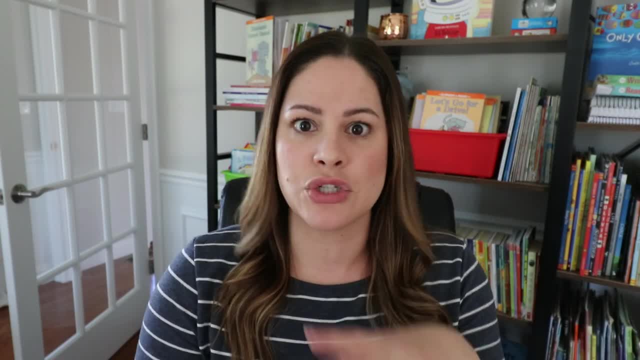 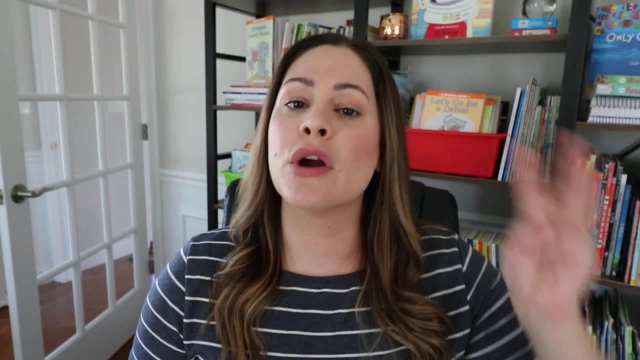 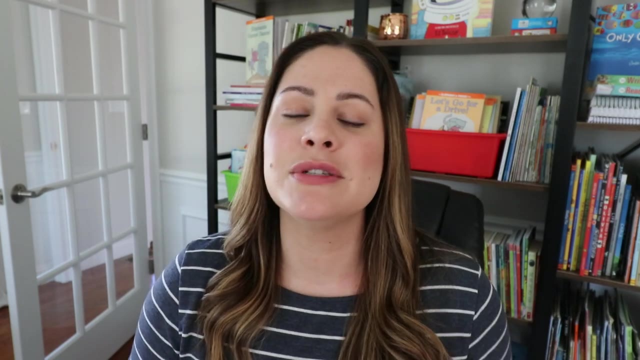 at counting up. So that's where you want to get them proficient in this skill right. You need to give them a lot of practice, And there are three games that I love to play that I'm going to show you right now that really help students get the gist of this. The first game I love students to play is called: 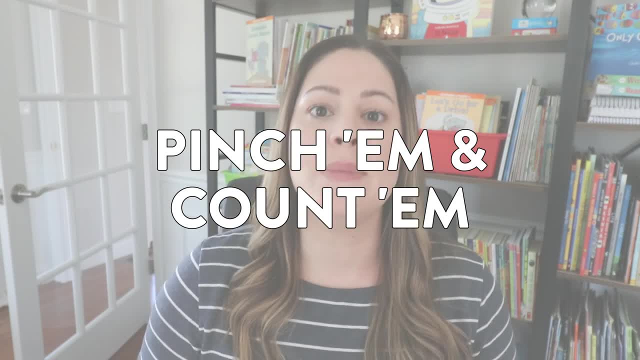 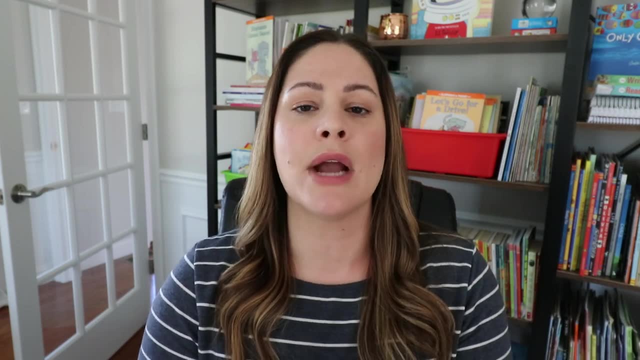 Pinch Em and Count Em, And this is a scaffolded activity because, instead of choosing a whole group of coins, like we were just doing, this independent practice has them practicing just counting up two different types of coins at the same time, And that's where you want to get them proficient in this. 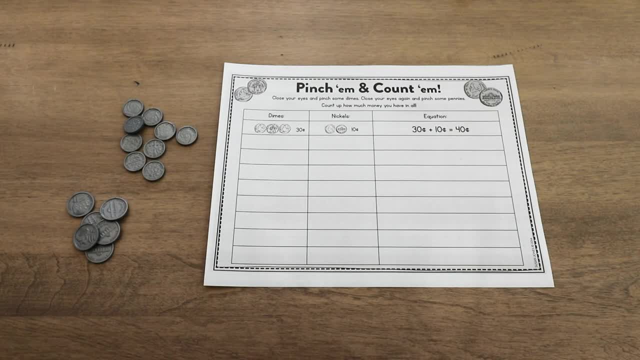 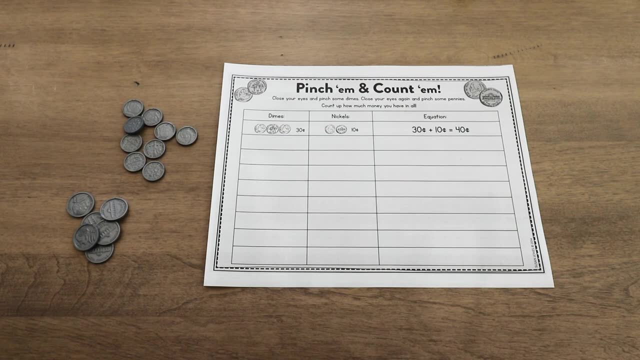 at a time. So, in order to do this, you will give students a pile of nickels and a pile of dimes. as an example Could be dimes and pennies, quarters and nickels- whatever- Two different types of coins. 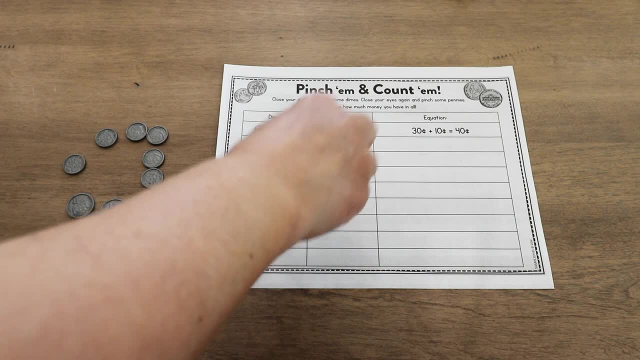 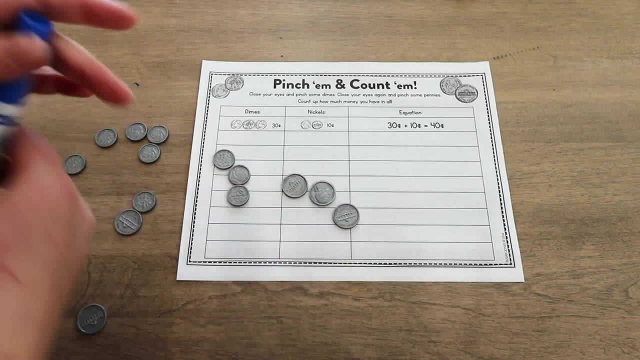 So once they have those coins, they will simply close their eyes and they'll just pinch some. So they're not taking a big handful, but they'll pinch up some nickels, drop them down on the table. Then they'll close their eyes and pinch up some dimes and drop them down on the table in front of. 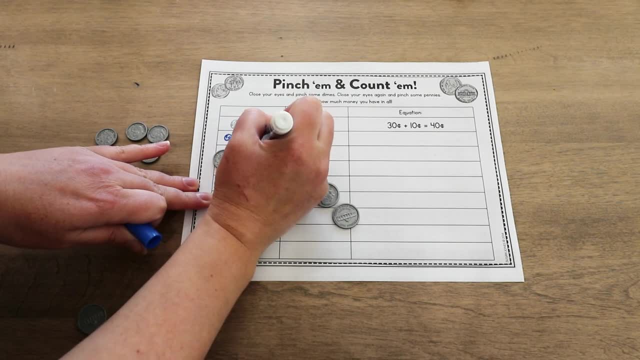 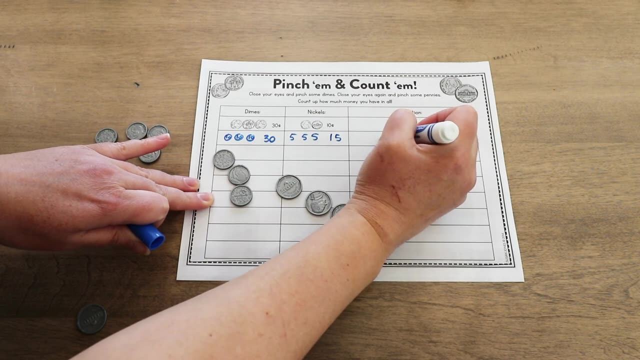 them. Once they've done that, they'll sort them if they are mixed together, And then they will write down on a sheet That looks like this one how many dimes they had and their value, and then how many nickels they had. 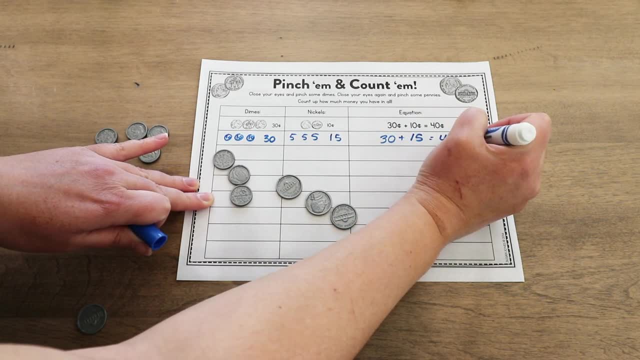 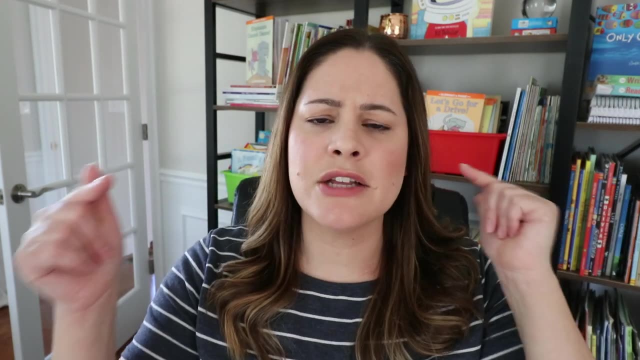 in their value. Then they'll go ahead and count them all up together to find the total value. Once they've done that, they will go ahead and put all their coins back, close their eyes, pinch them, count them, add it up again And, as you can see on that sheet, I think they would do this about 10. 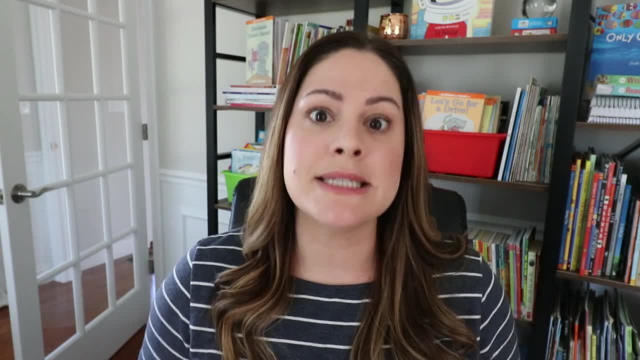 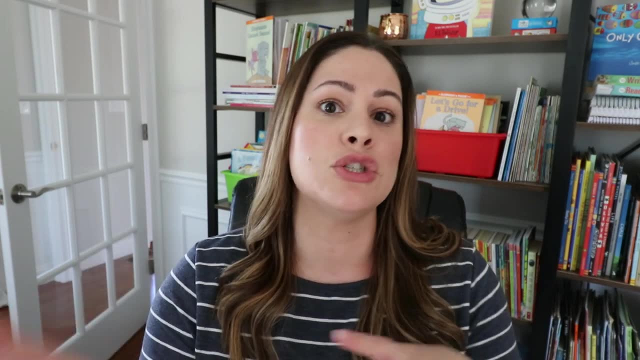 times. So it's a very simple way for students to just practice getting those coins together, sorting them, counting them up and really knowing those values, And it's super easy to switch out by picking two different coins each time. The next money game I love to play is a great one to get students noticing both the top and the. 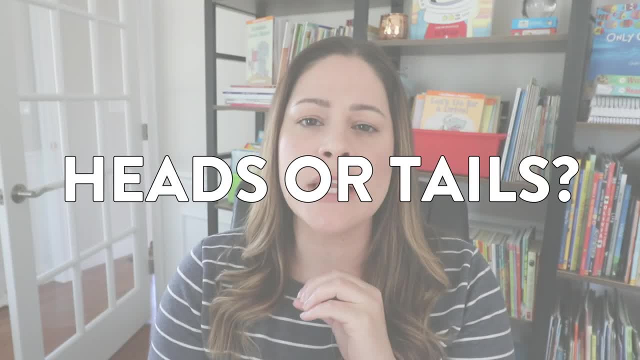 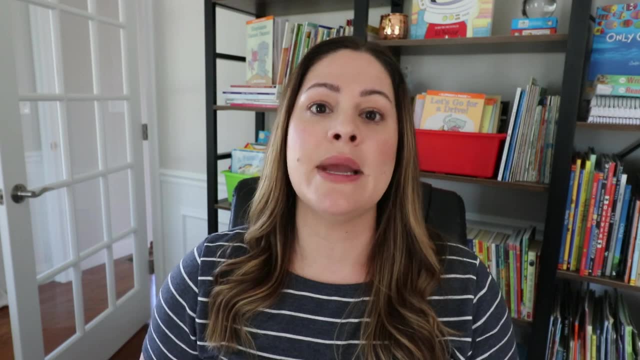 bottom of the coin. Sometimes the back of the coins are a little trickier for some kids, and other times it's the front of the coins are trickier because the heads all look the same. But for this one, all students are going to do is you can start with a same group. So let's grab a group of nickels. 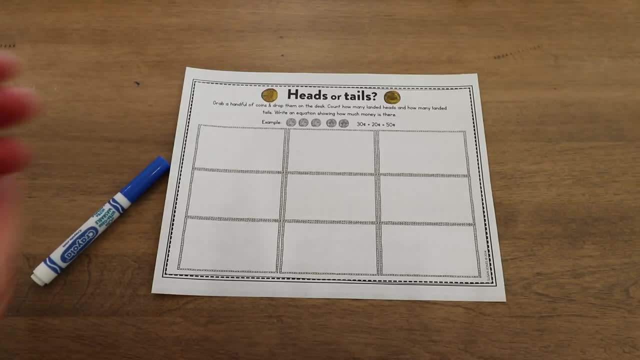 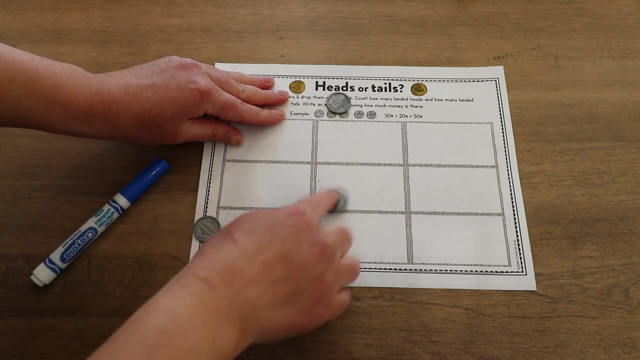 and students will grab a handful, or again a pinch, because we don't want them having too many at one timebut they'll grab some of those nickels and just drop them on their table. It's called a push Then, instead of sorting by type, because they're all nickels, they will go ahead. 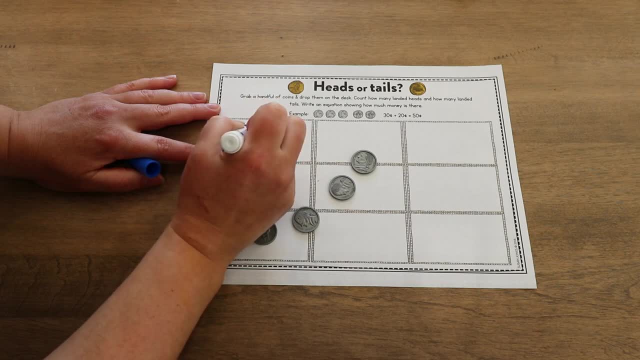 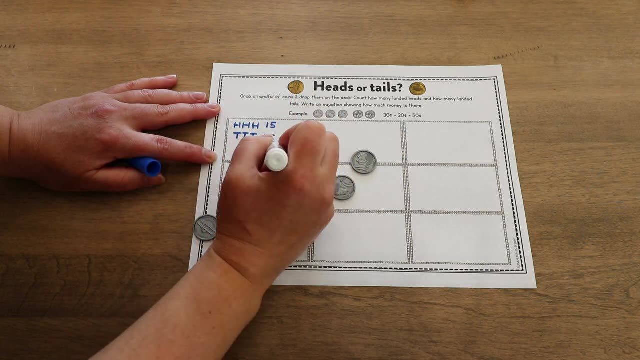 and sort them by which one landed on their head and which one landed on their tails. Once they've gone ahead and sorted them, they will write a little addition equation counting up the value of coins that landed on their head and the value of coins that landed on their tails to find out the total value. You can see. 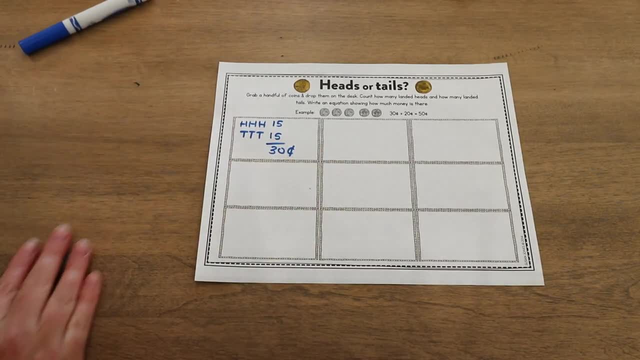 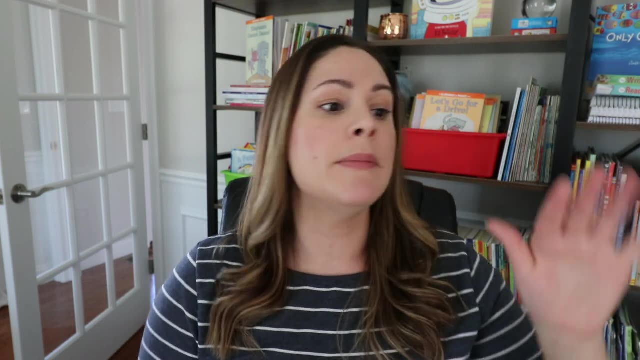 that little recording sheet has them do this about nine different times, and I love this activity because you can completely differentiate this for all of your students So they can play all the same game. but maybe some students are just working on pennies or they're just working on nickels and maybe some of 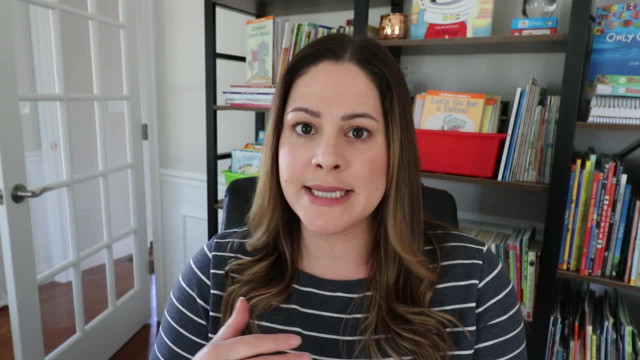 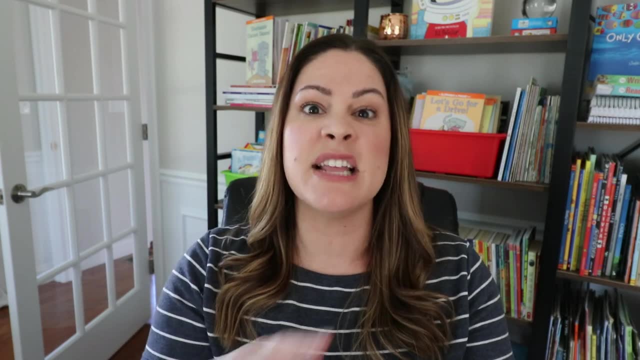 your other students are ready to really start counting up those mixed coins again. and practice that, and they can just grab a group of mixed coins. do the same thing and they'll sort them by heads and tails and they'll have to count up two different groups of mixed sets for all the ones that landed on. 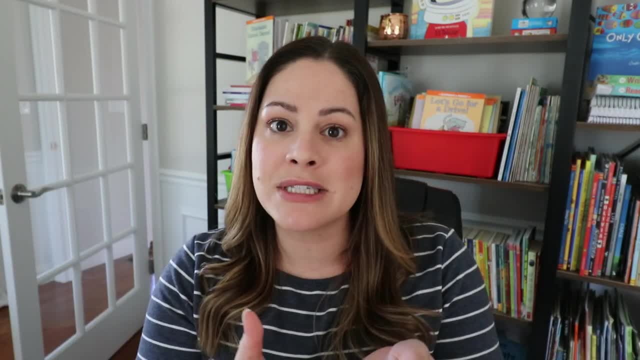 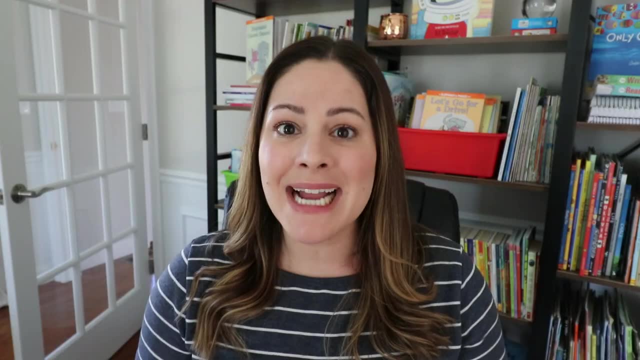 their heads, all the ones that landed on their tails, and then add those together to find the value as well. The last game I love to play is called Pop the Piggy, and I'm not actually going to explain how to play it right now, because 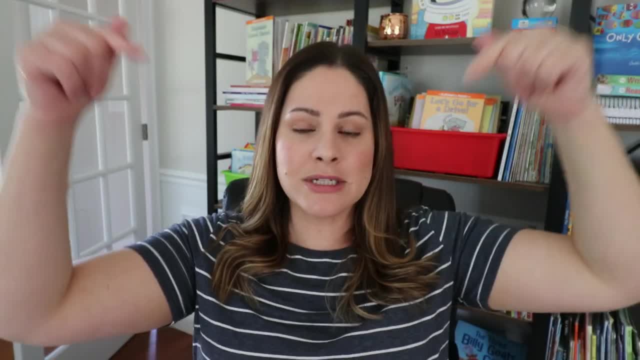 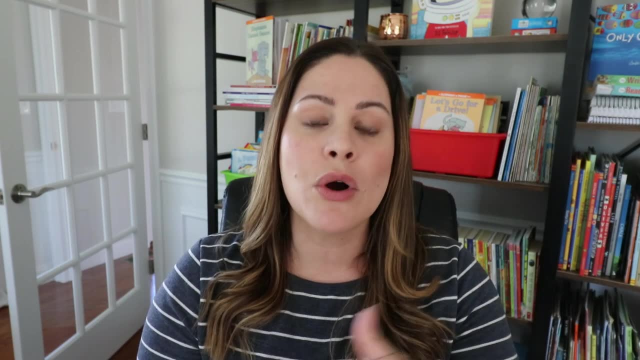 I did a whole video and made a complete freebie. It looks like this right here, so I will link that and I'll put a little card here in this video so at the end of this you can go over to that. It's a quick video that shows how to play the. 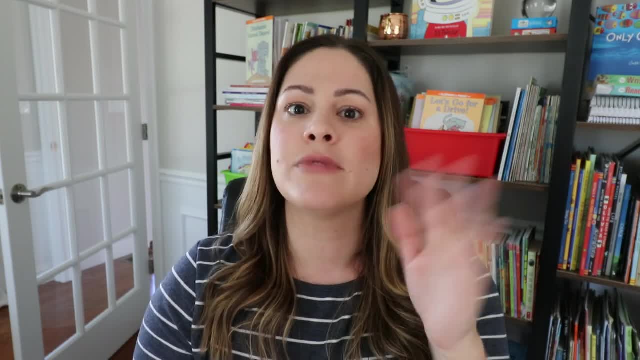 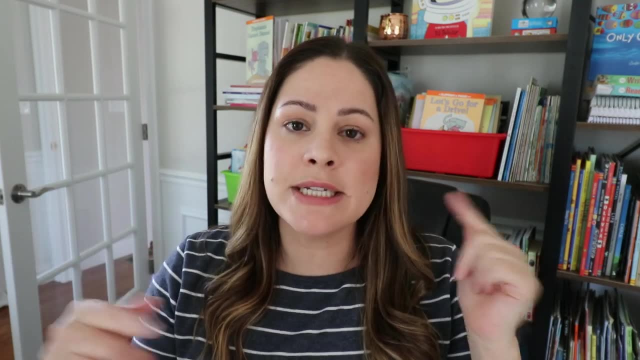 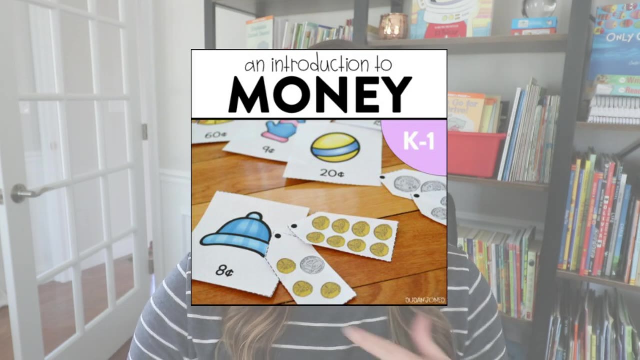 game and it has all of the printables, directions and everything that you can just print out and grab over there And- just a little side note, all of the anchor charts and the little worksheets and everything I've shown so far in this video and also the money unit is a little bit different than the憂mouh unit. 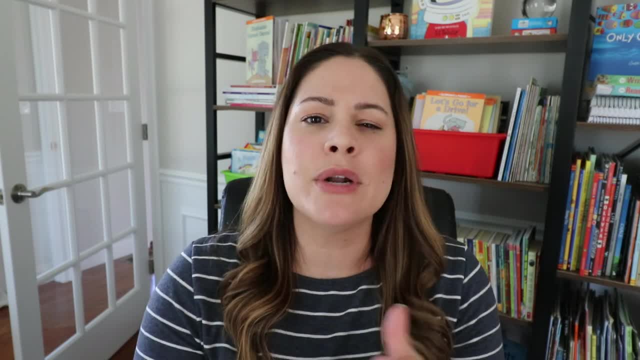 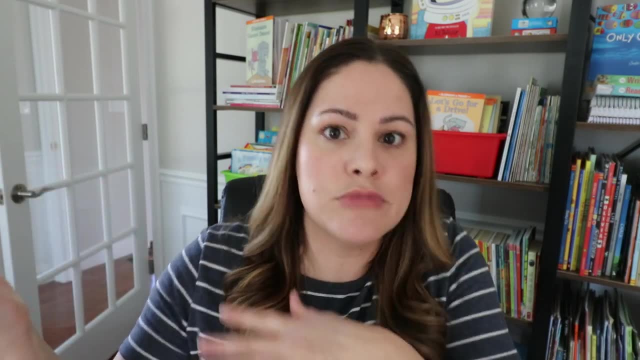 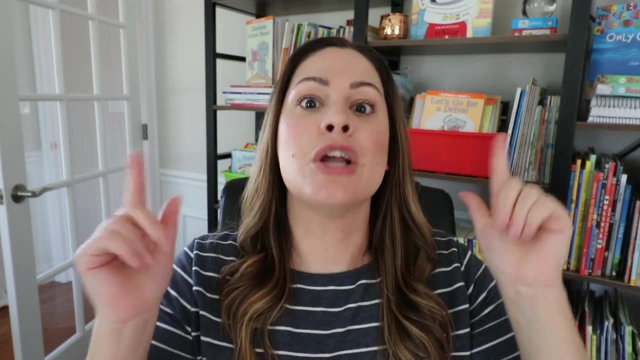 right here on TPT. It's my introduction to money unit and it has way more activities than the ones I'm sharing in this video, but I wanted to share a couple, like heads and tails and pinch them and count them, that you don't actually necessarily need those sheets to be able to play, So that way you can. 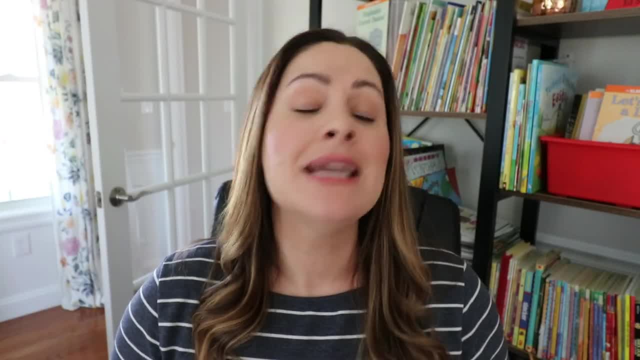 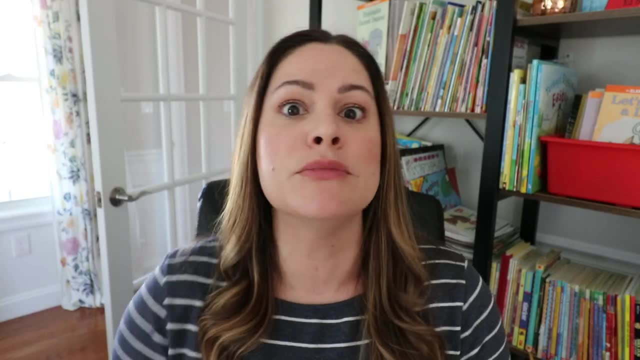 take these activities and use them in your classroom, but if you are looking for a lot more, go ahead and check that unit out. Okay, step number four: when teaching, Money is one of those concepts that very quickly and very easily becomes real life right, Even if they're not using coins as much anymore. 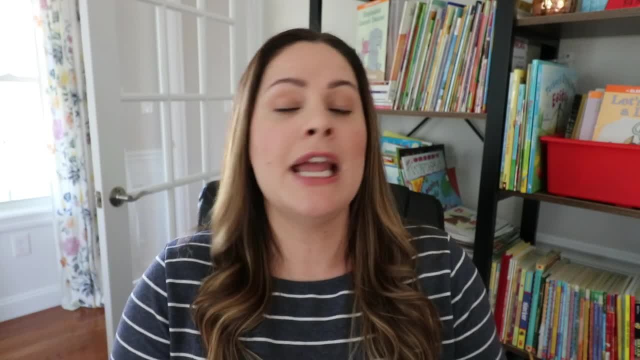 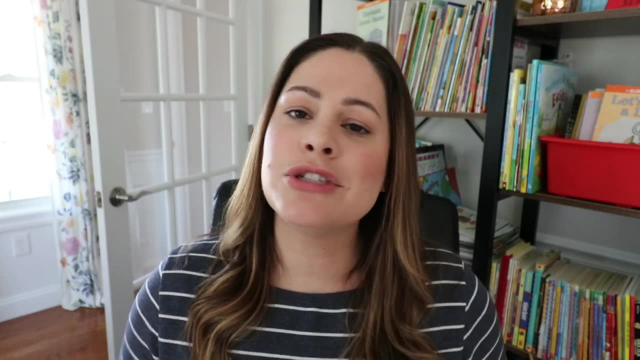 and they're really using debit cards, they still need to be able to figure out if I have enough money in my bank or in my pocket or in my wallet to be able to purchase something, And in order to do that, I really like to use some story problems. 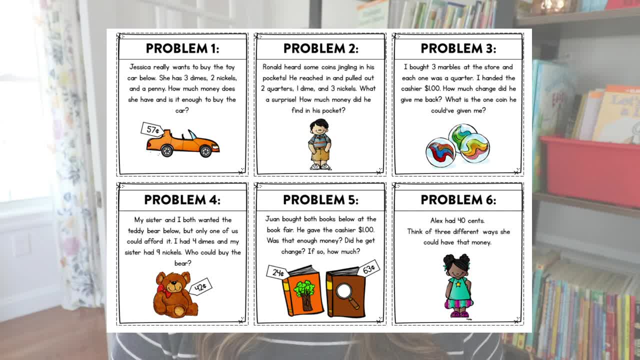 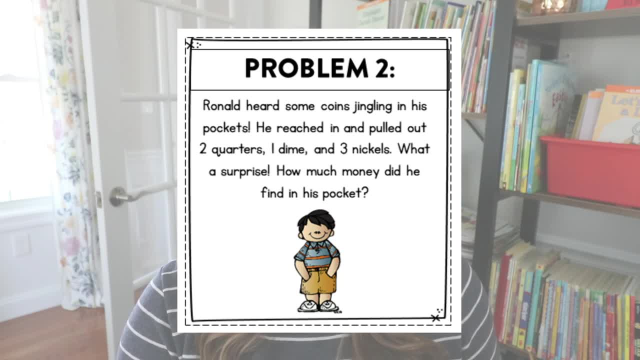 that look like this to get students really thinking about money. Here you can see a few different ones. Problem number two says Ronald heard some coins jingling in his pockets. He reached in and pulled out two quarters, one dime and three nickels. 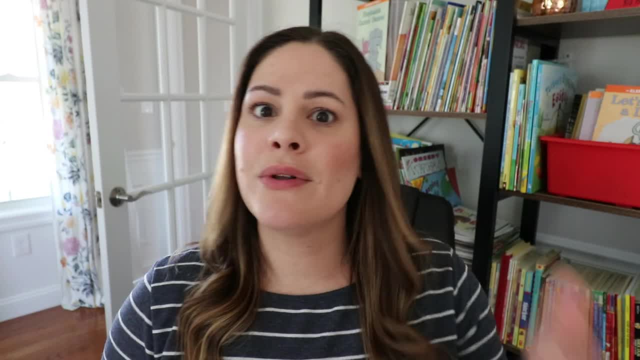 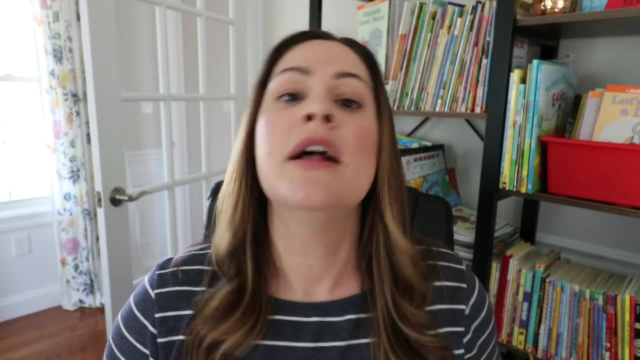 What a surprise. How much money did he find in his pocket? So this one is just like: oh a fun surprise, He had this many things. Count up how much money he had, but it's in a word problem format. Another type of problem you might wanna ask is like this: 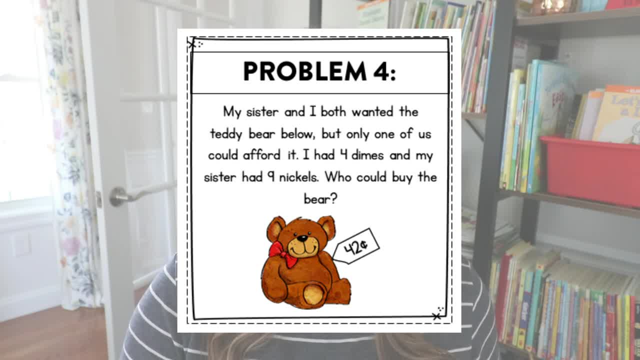 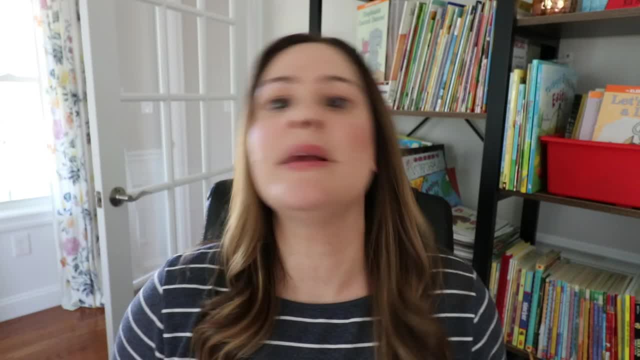 My sister and I both wanted the teddy bear below, but only one of us could afford it. I had four dimes and my sister had nine nickels. Who could buy the bear? So this is a great one because students can see that bear. 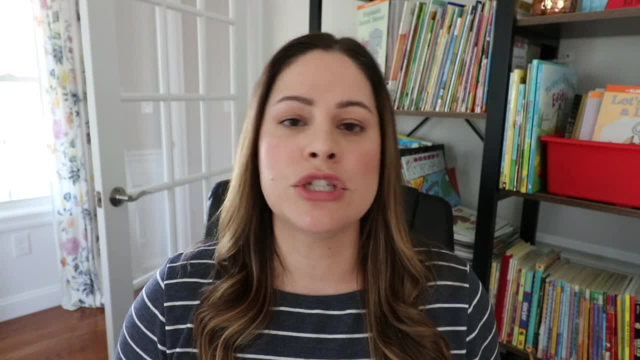 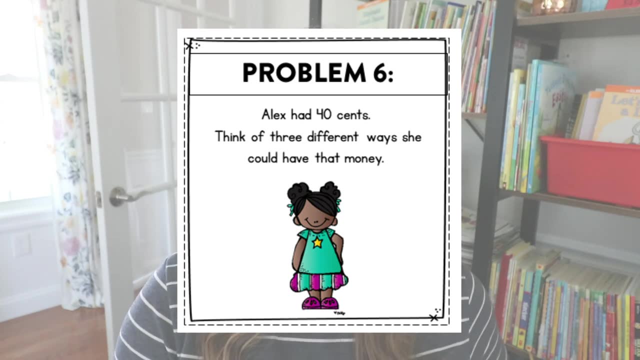 and it says it's 42 cents. They have to figure out which sister can actually afford and has enough money for the bear. And for another example, problem six, says Alex had 40 cents. Think of three different ways she could have that money. 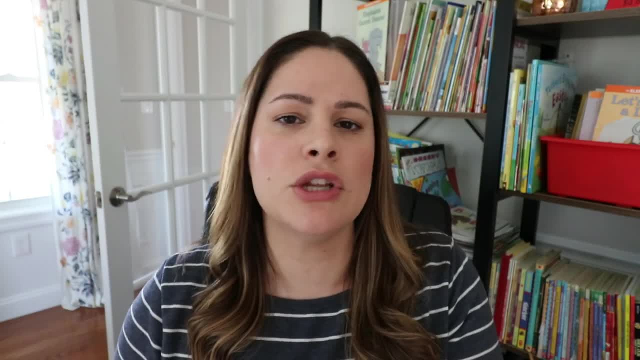 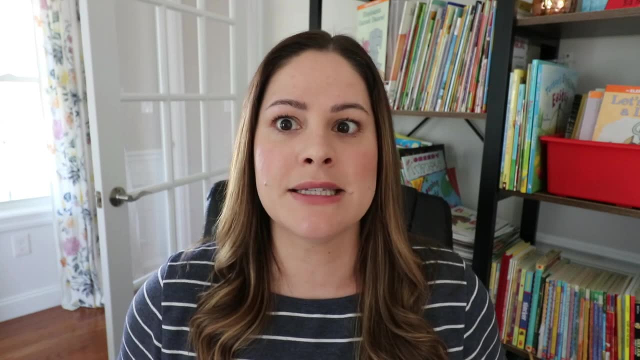 And this just gets students thinking about different configurations that they could use of the coins. So it helps them really think of their coin knowledge and value knowledge. to figure out three different ways she could have 40 cents. Those were just three quick examples of different types of word problems. 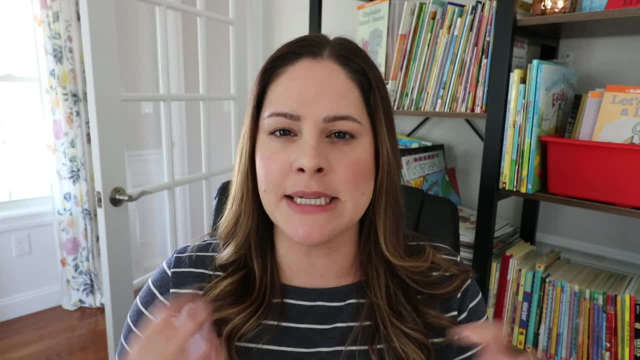 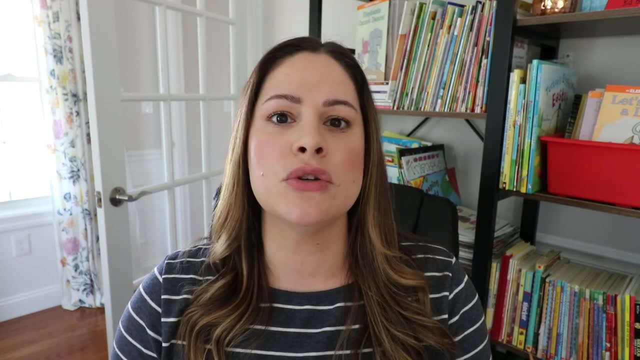 you might want to pose to your students, because it gets them thinking about money in slightly different ways. Feel free to go back to that slide and pause and take a look at the different problems I shared there. Each one gives students a different way of thinking about money.